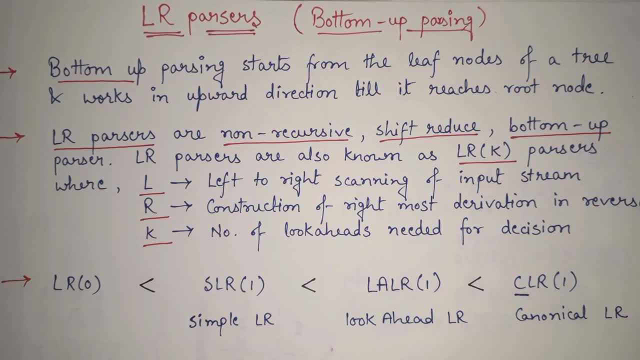 recursive descent parser, predictive parser, operative precedence parser- We have already seen those. Now we are supposed to start one of the most important category of parsers in compiler design, that is, LR parsers. First of all, as I have already discussed, we are having main four types of LR parsers. 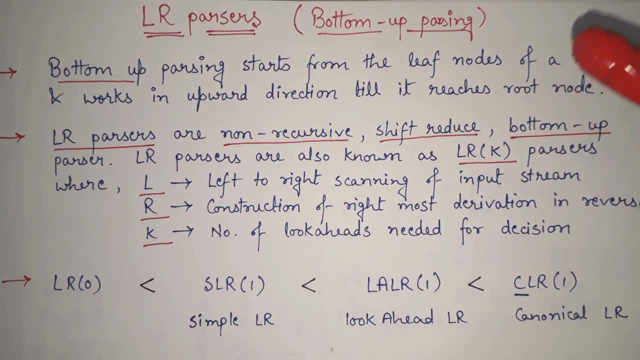 that is, LR0, SLR1, CLR1 and LLR1.. These are the four main types of LR parsers that we have to learn. But before directly going into the parsers, you must have an overall idea that what LR parsers are. 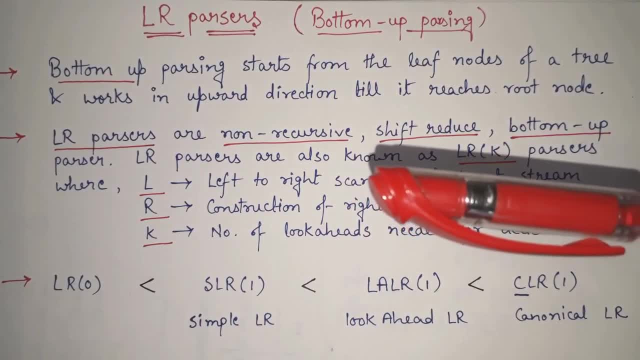 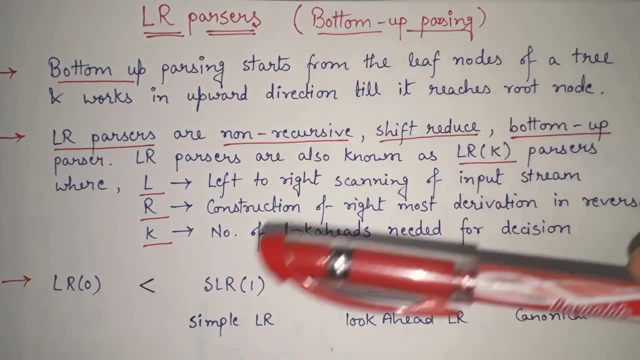 As I told, this is really a very important topic, So let's not skip anything. First of all, let's clear, Let's get a clear idea that what are LR parsers, and then we can go in detail of each individual parsers and we will see respective examples also. 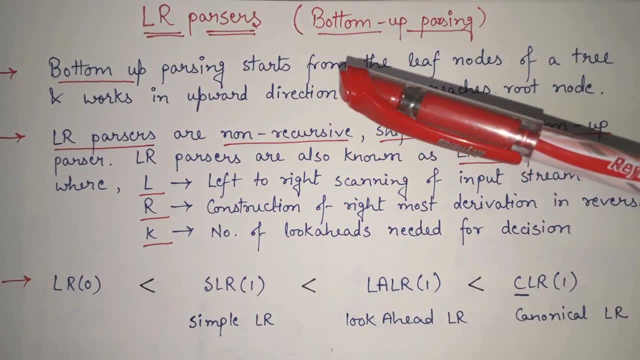 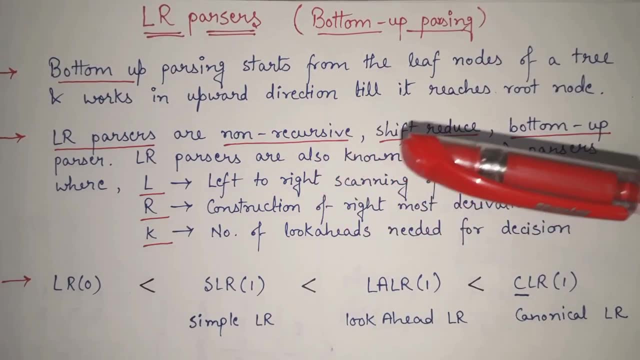 So, first of all, what are LR parsers? They are coming under the category of bottom-up parsing. They are bottom-up parsers. As we have seen, the two broad categories are top-down parsers and bottom-up parsers. In the bottom-up parsers, the first category was operative precedence parser. 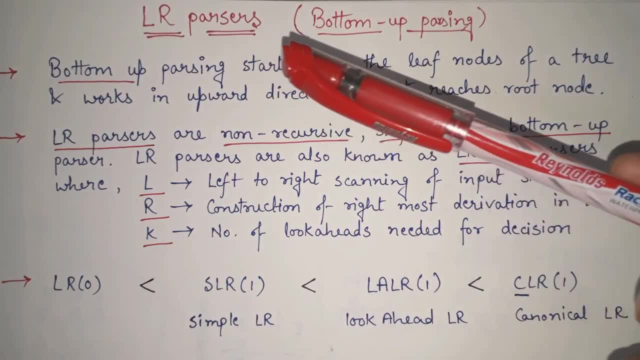 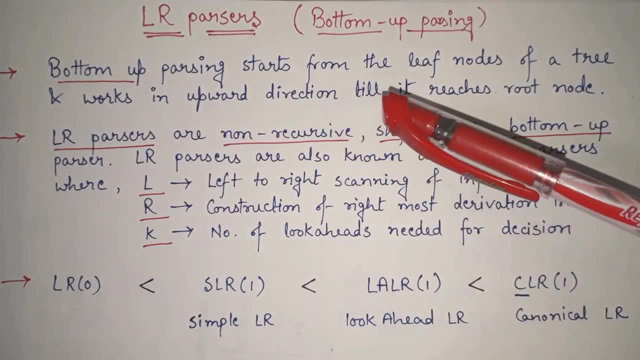 and the second category consists of all these LR parsers. Now, LR parsers are bottom-up parsers, As the name itself indicates. what do we mean by bottom-up parsing? Bottom-up parsing starts from the leaf node and works in upward direction till it reaches the root node. 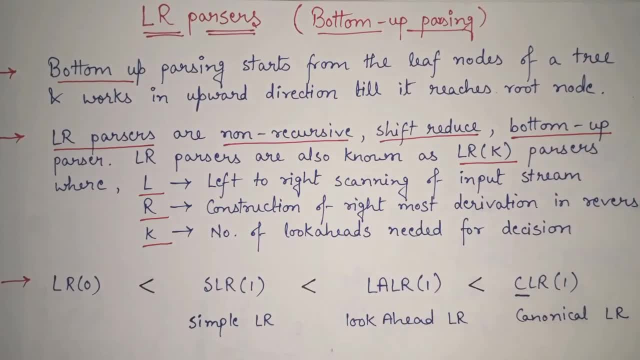 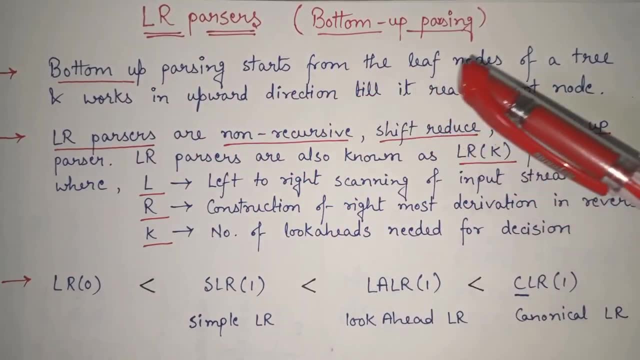 As the name itself indicates, bottom-up parsing starts from the leaf node, starts from the bottom and reaches up to the top. So bottom-up parsing starts from the leaf node of the tree and works in upward direction until it reaches the root node. 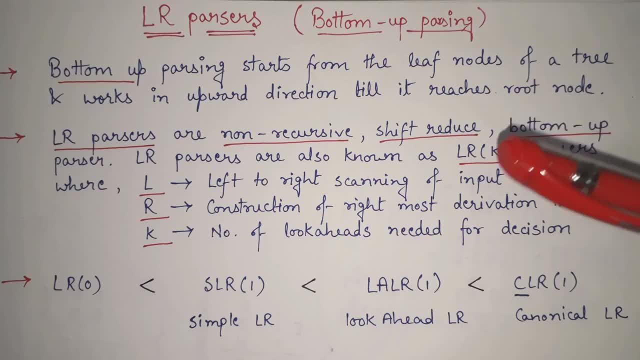 Fine, Why I am telling you all these things? So that you will get a clear idea. So let's get started. You will get a clear idea what LR parsers are And, apart from that, first of all, your concepts will be clear. 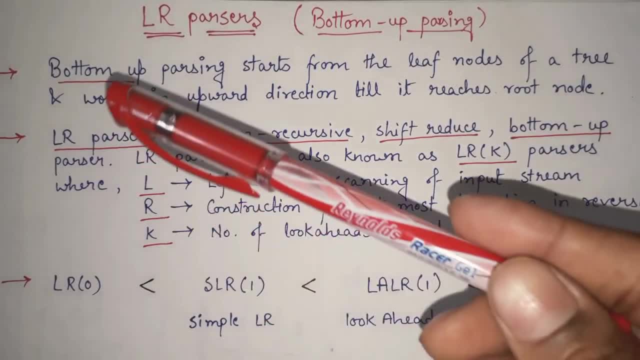 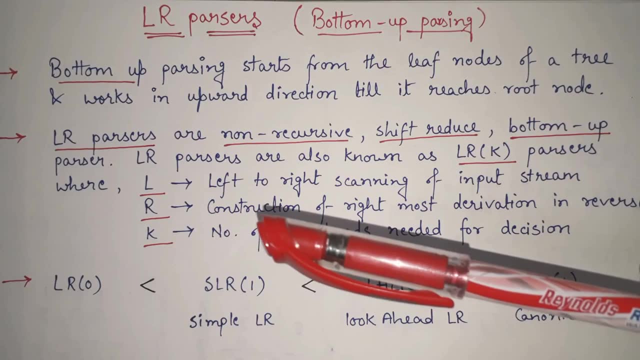 And apart from that, in many of our BTech, MTech exams also, these are the common definitions. These two, three things are very common that are being asked in one-two mark questions. So you must be aware of these things. 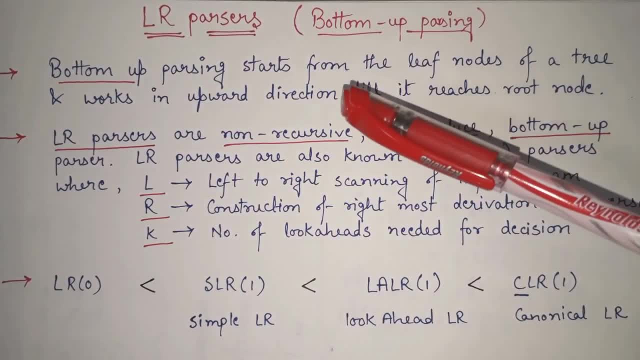 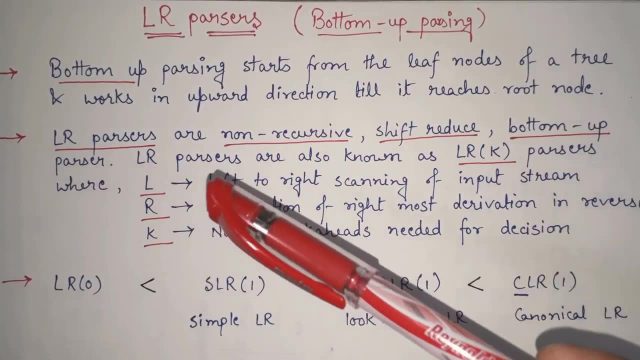 Fine. So first of all, why it is known as bottom-up parser. We have already seen Now what exactly LR parsers mean. Why do we call them LR parsers? So LR parsers are nothing, but they are non-recurrent. 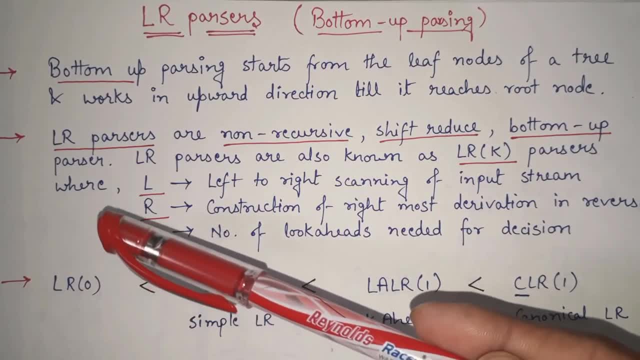 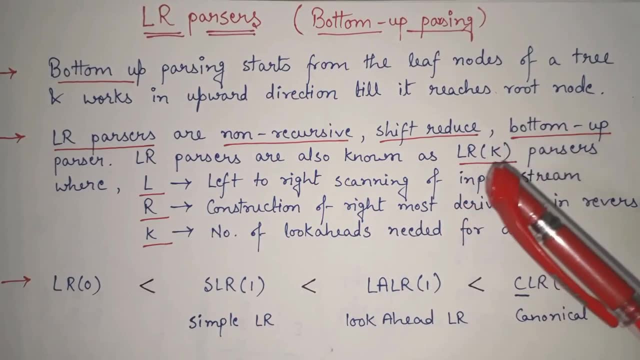 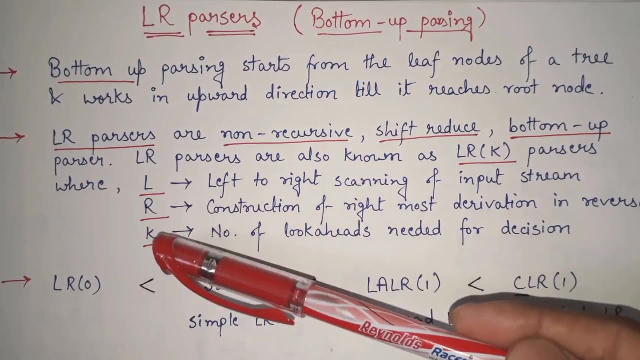 They are recursive shift-reduce bottom-up parser. LR parsers are also known as LRK parsers, LR and see, note it down- LR, and inside bracket we are having K- They are also known as LRK parsers- where now again, this is one of the most important thing, that in LR parsers particularly, what does this L and R mean? 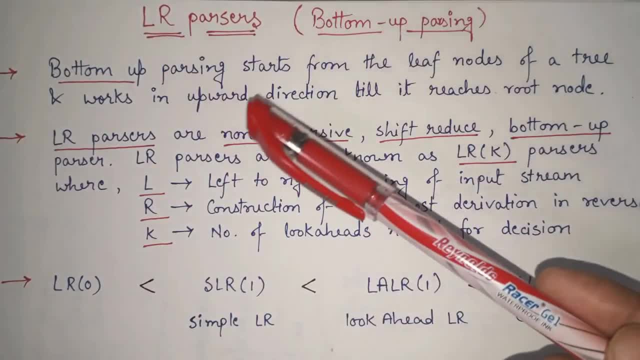 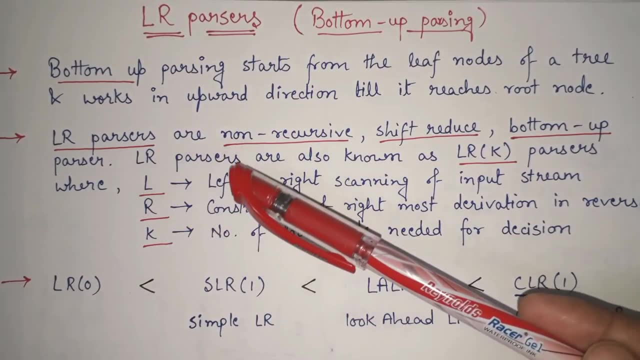 Many people are not knowing this. They are knowing the whole examples of LR parsers but they don't know even what is L and what is R. Right, But we must be knowing that. So what we have written, that LR parsers are also known as LRK parsers. where LRK? what do they mean? 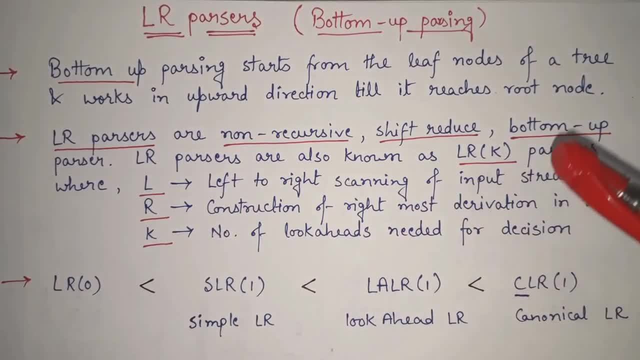 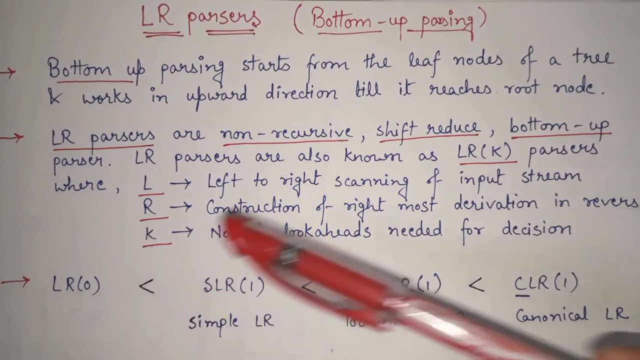 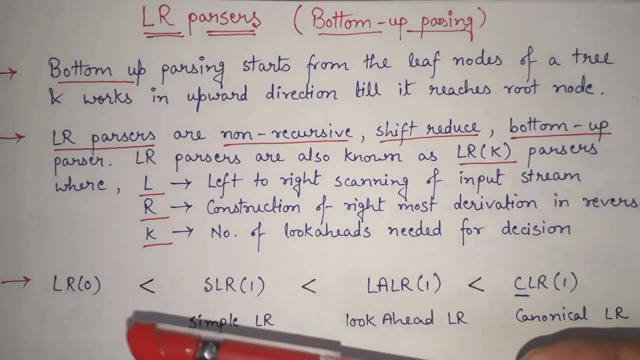 L means left to right scanning of our input stream. R means construction of rightmost derivation in reverse. And this K, that is inside this bracket, this K means number of look-aheads needed for the decision. Now, what exactly are look-aheads? 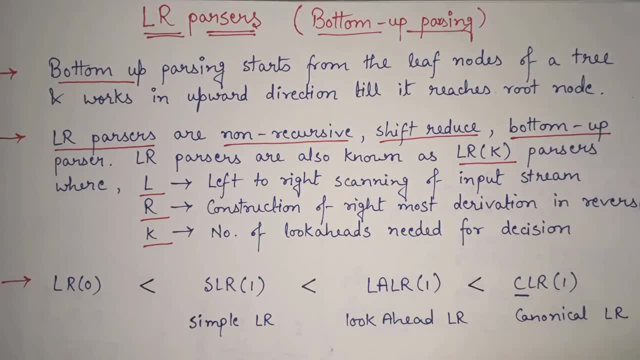 We will see as we proceed. We will see as we proceed in our examples. Fine, But these are really very important things that you must be knowing. What is L, What is R? These two questions are something that has been asked multiple times in competitive exams also. 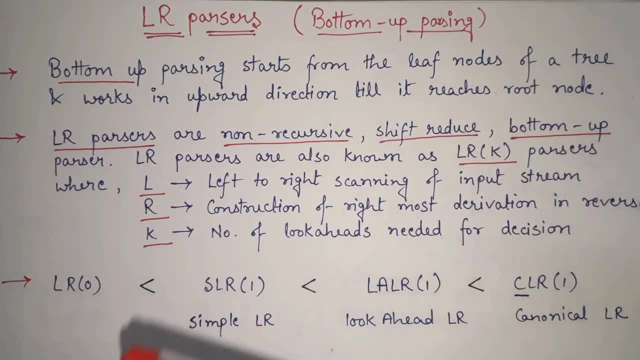 So this is. I have collected here some of the important definitions so that you can note them out and you can refer whenever required. So these are basically what L, R and K means. Now, as we have discussed, the four main types of LR parsers are LR0, SLR1, LLR1 and CLR1. 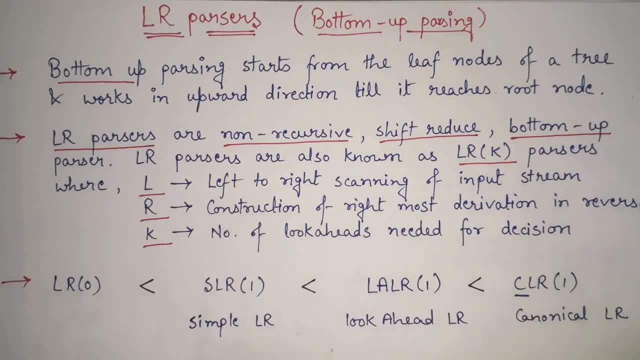 LR0, what is LR? We have discussed the full form of LR. Then SLR means simple LR, LALR means look-ahead LR And CLR means canonical LR. These are the four main types of LR parsers. Now, if we talk about, we will, we will be seeing all these term, all these terminologies and all these parsers in detail in the coming video. don't worry about that. 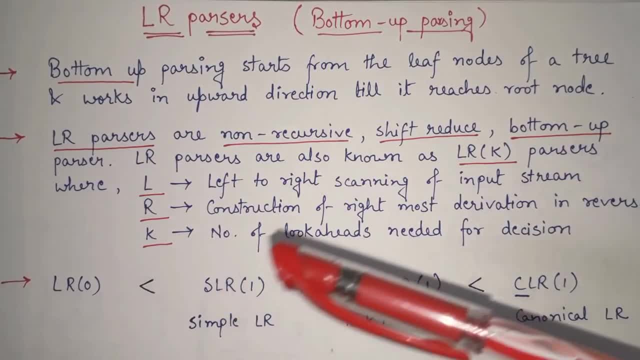 But in this video I just want to give you some important definitions and just an overview. But in this video I just want to give you some important definitions and just an overview. Now, if I see in a broad category that what is the main difference between these four? 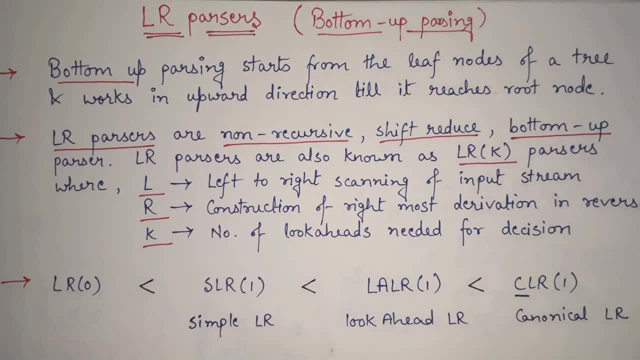 So the main difference is see, if we talk about in terms of power, then among these four, CLR1 is considered to be most powerful. Fine, So it is also a common question that what is the most powerful LR parser? 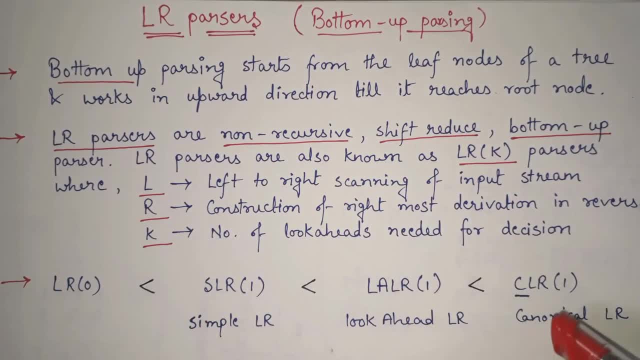 So, among all these four, the most powerful LR parser is CLR1.. This is written in the in the order of LR. This is written in the in the order of LR. This is written in the in the order of LR. 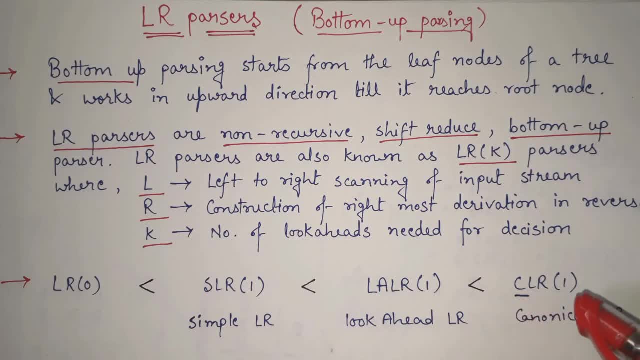 This is written in the order of LR. This is written in the order of LR: See CLR1. parser is most powerful. See CLR1. parser is most powerful. After that we are having LALR1,, after that we are having SLR1, and after that we are having. 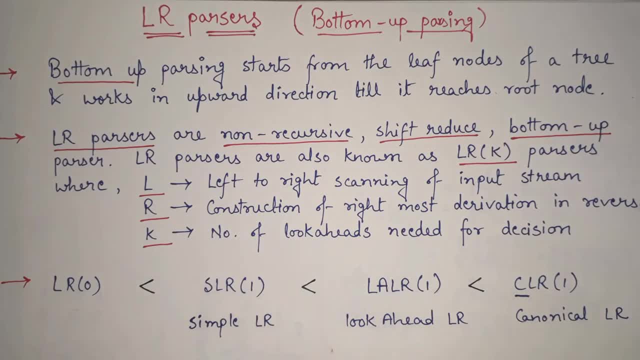 LR0.. In LR parsers, we can say that LR0 is the least powerful one. In LR parsers, we can say that LR0 is the least powerful one. Now, yes, one more thing, that CLR 1 parser, CLR 1. many times it is also known as simple. 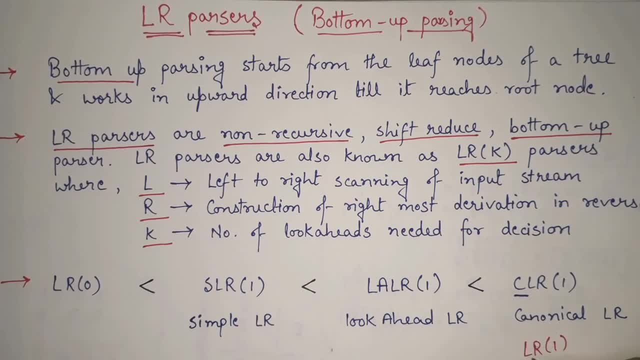 LR1. So in exam, because this small, small things are very important to know, otherwise it can it can cause a big loss. many times, in example, LR1 is asked. if we don't know what is LR1, then you cannot solve it, though you know how to solve CLR1, so these are important things. 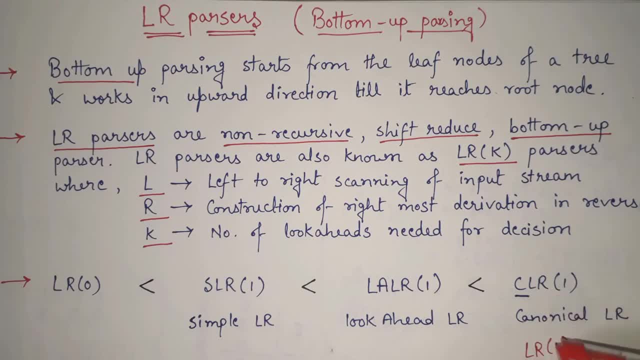 so you should be knowing that if in any question LR1 is written, LR1 is nothing, but it is same as CLR1, so many times CLR1 is also known as simply LR1,. so yes, these are the four main LR parts. this is the order of their power and apart from that, what yes here? see if you. 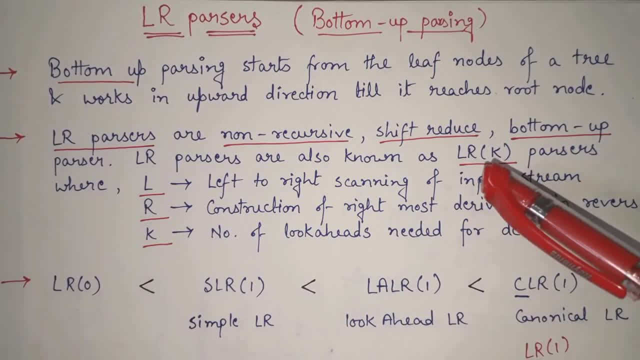 note here. this is inside the bracket that is K, the value of, as we have seen. what is K? K is the number of lookaheads needed for the decision. so this K. you have to remember that the value of K in LR0 is 0, but apart from that, in all these three we are having the value of K as 1, now. 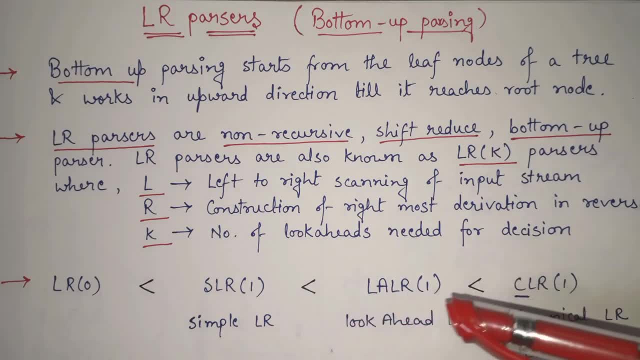 why it is known as canonical LR, why it is known as lookahead LR, what our lookaheads? we will see all these things in the respective videos. fine, we will be seeing now. this is just an overview. I just wanted to highlight the important points that you have to. 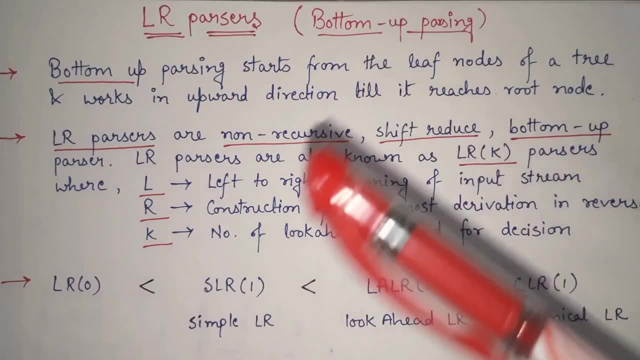 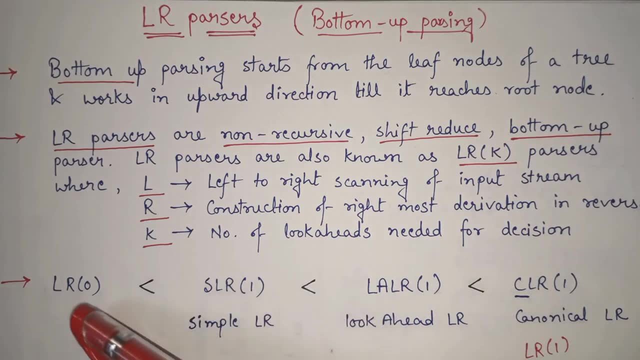 remember the important questions that are being small, small theory questions that are being asked. we wanted to inform you people that one. now we will be starting particularly all the four, all the four parcels. we will be seeing that how they are the main difference between these four.